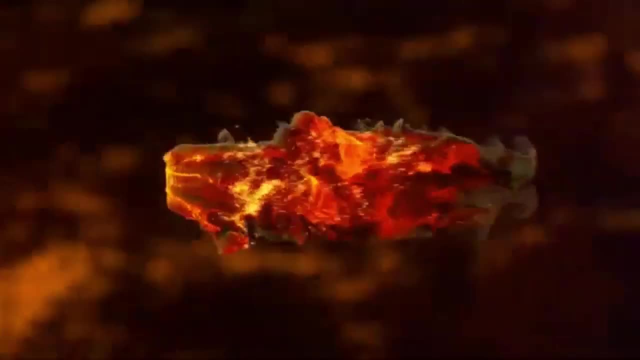 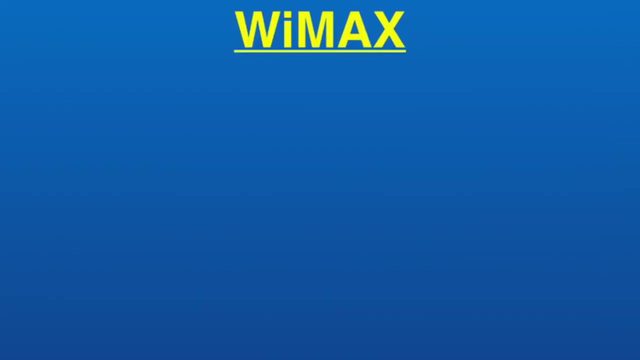 Hello everyone. Today we are going to talk about. WiMAX Stands for Worldwide Interoperability, for Microwave Access, and it is a technology for point-to-point and point-to-multipoint wireless connection. WiMAX technology is a wireless broadband communications technology based on IEEE 802.16 standard, providing high-speed data over a wide area. It was 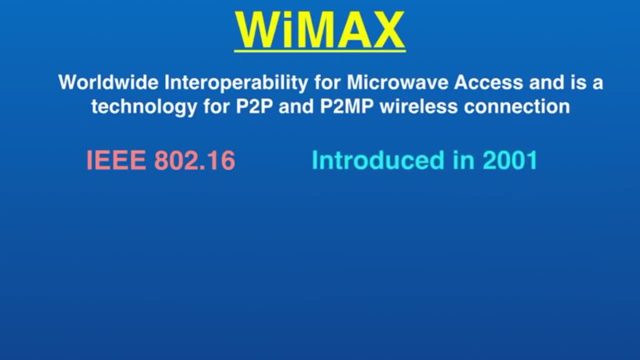 introduced in 2001.. WiMAX wireless microwave access technology can provide 4G levels of broadband wireless access for both mobile and fixed applications. It was considered a prime candidate for 4G mobile networks over CDMA, GSM and HSPA. 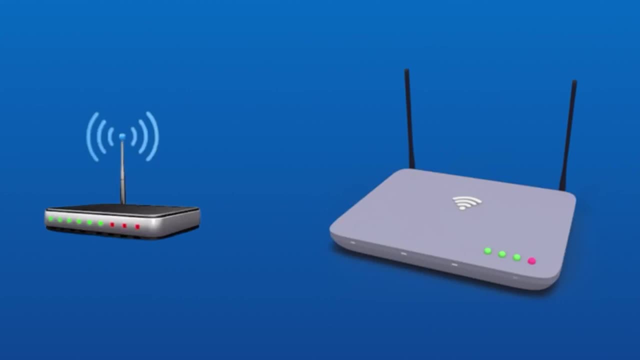 Being a part of 4G wireless communication technology, WiMAX has surpassed the 30-meter wireless range of a traditional Wi-Fi local area network, offering a metropolitan area network with a signal radius of about 50 kilometers. WiMAX was originally proposed as a wireless 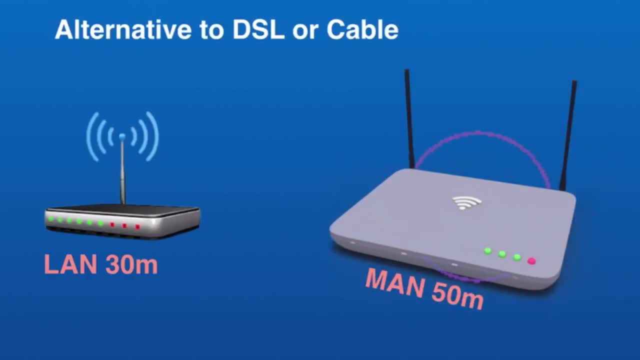 alternative to wired internet access at the time, particularly in areas that are difficult for wired infrastructure to reach, and the ability to overcome the physical limitations of wireless communication technology. WiMAX works similar to Wi-Fi, but at higher speeds Over greater distances. WiMAX provides. 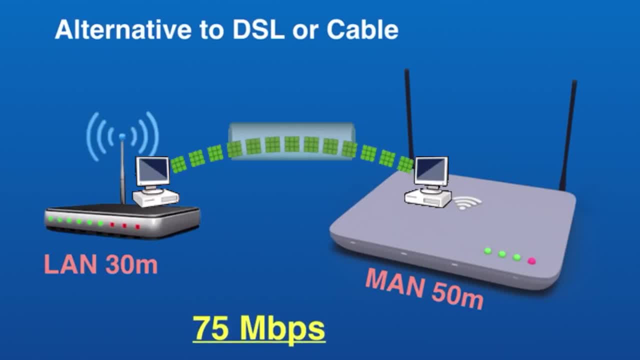 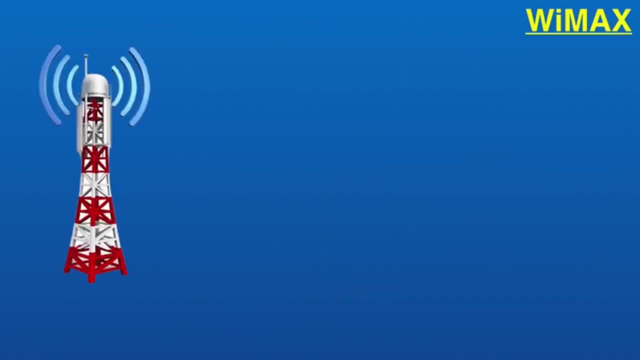 data transfer rates of up to 75 megabits per second, which was quite superior to conventional cable modems and DSL connections. WiMAX operates over radio waves On a tower-receiver model. a single WiMAX tower can provide coverage over about 8,000 square kilometers. WiMAX is a multi-modal, multi-division, multi-tower. 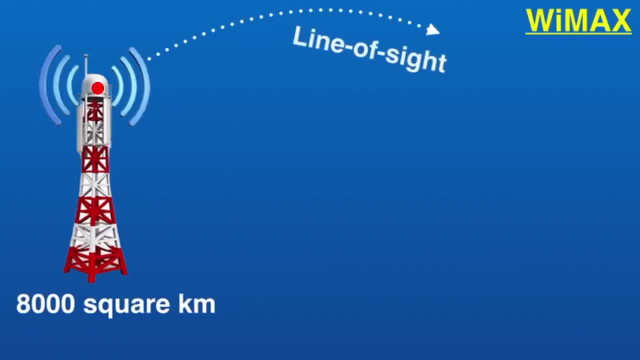 multi-vibration network. WiMAX networks are now much more stable and efficient With WiMAX square kilometer and also connect to the other towers via a line of sight microwave link to expand coverage. further line of sight communication means when there is no signal obstruction between transmitter and 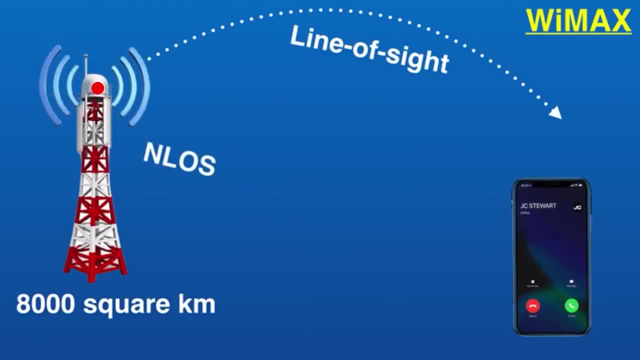 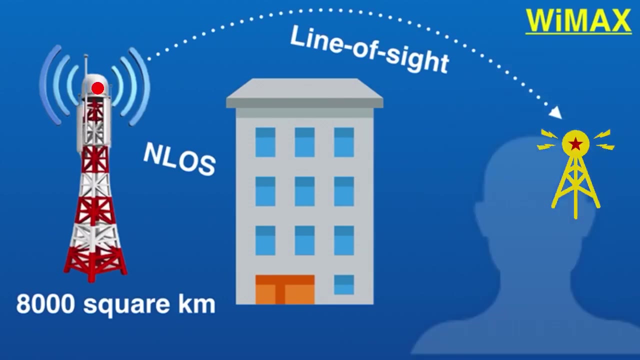 receiver. non line of sight communication is also possible even when there is a signal obstruction between transmitter and receiver. signal arrives at the receiver after going through many reflections in between. why max technology is proficient to meet the needs of a large variety of users from those in developed nations who want to install a new high-speed data network. 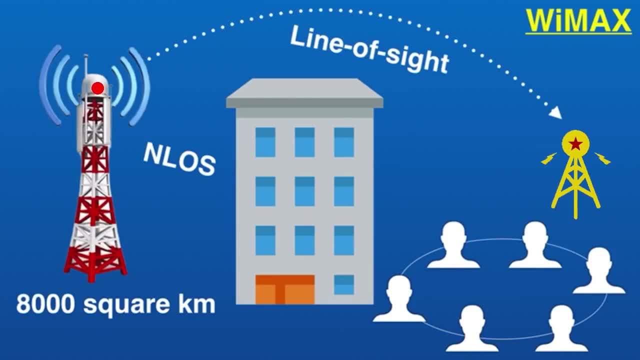 very cheaply, without the cost and time required to install a wired network. to those in rural areas who need fast access, we are wired solution may not be possible because of the distances and costs involved effectively providing WiMAX broadband. additionally, it is being used for mobile applications providing high-speed data to users on. 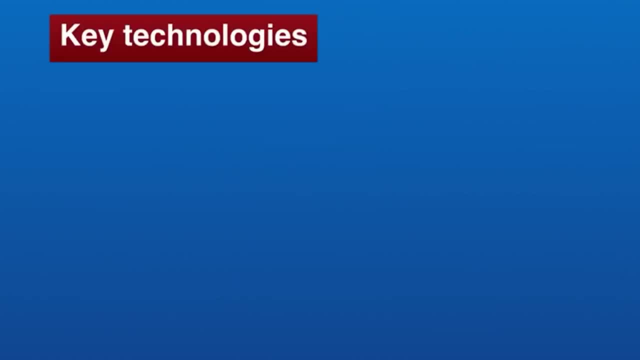 the move. WiMAX broadband technology uses some key technologies to enable it to provide high-speed data rates: OFDM, orthogonal frequency division, multiplexing, OFDM- has been incorporated into WiMAX technology to enable it to provide high-speed data without the selective fading and other issues of 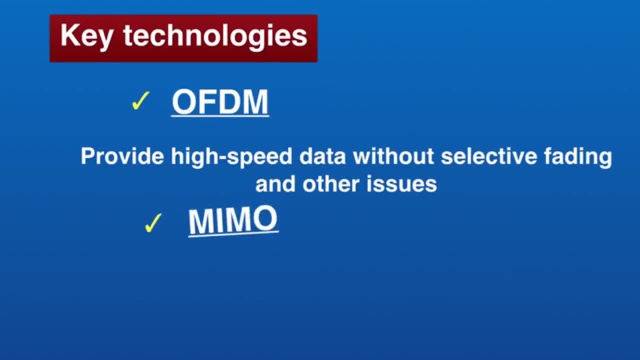 other forms of signal obstruction: MIMO, multiple input, multiple output. WiMAX technology makes the use of multi-path transmission using MIMO. by utilizing the multiple signal paths that exist, the use of MIMO either enables operation with lower signal strengths levels are allows for higher data rates. 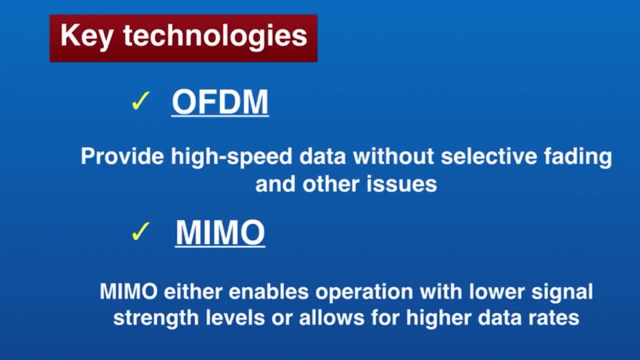 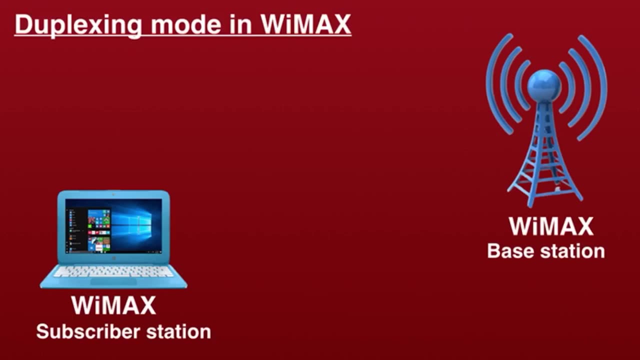 WiMAX and Wi-Fi are complementary. while WiMAX is a broadband connection to the internet at service point, WiMAX and Wi-Fi is a wireless local area network. duplexing modes: in Wi-Fi duplexing means the way downlink and uplink data is arranged in a two-way. 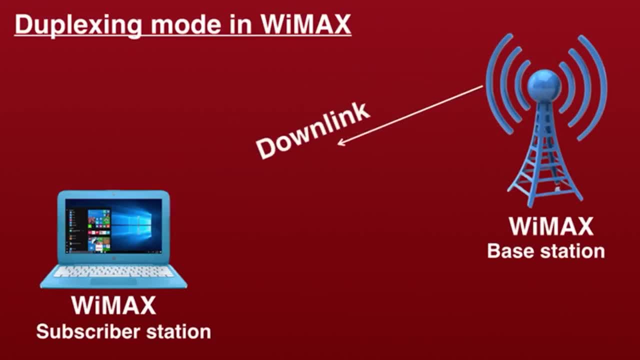 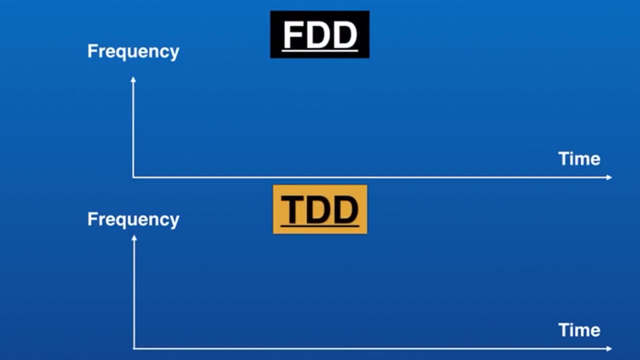 wireless transmission. downlink carries information from a base station to subscriber station. downlink is also known as a forward link. uplink carries information from subscriber station to base station. it is also called reverse link. There are two types of duplexing modes: FDD and TDD. frequency division: duplex requires 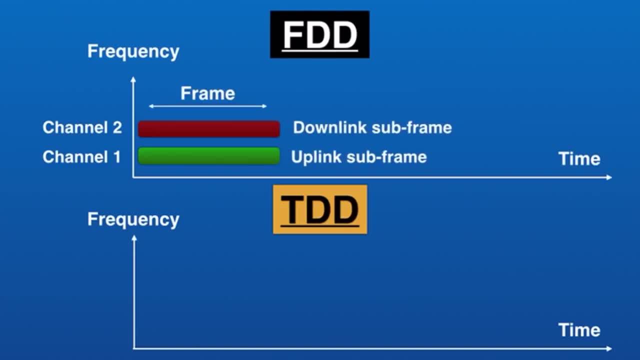 two distinct channels for transmitting downlink subframe and uplink subframe at the same time. slot FDD is commonly used in 2G and 3G mobile networks, WiMAX, sports, full duplex FDD and half duplex FDD. FDD is inefficient for handling. WiMAX supports full duplex FDD and half duplex FDD. FDD is inefficient for handling. WiMAX supports full duplex FDD and half duplex FDD. FDD is inefficient for handling. WiMAX supports full duplex FDD and half duplex FDD. 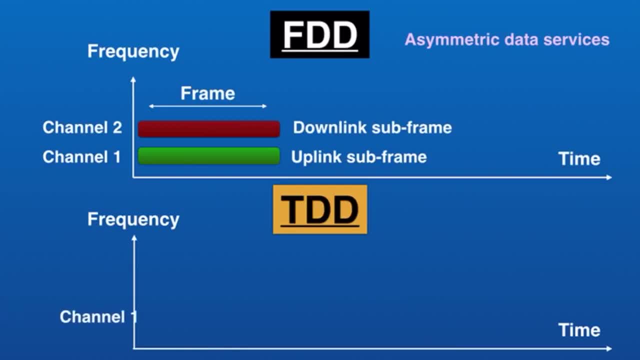